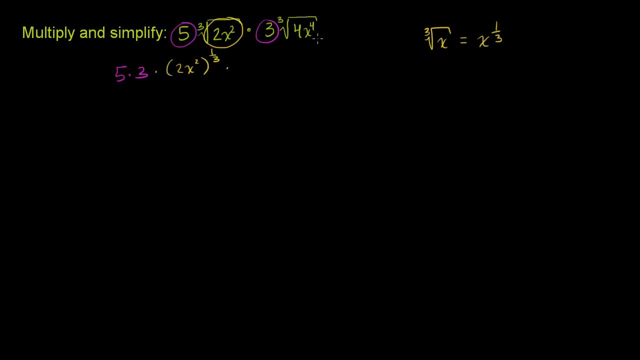 to the 1 third power. And then I have the cube root of 4x to the 4th, So that's the same thing as 4x to the 4th to the 1 third power. And now we know from our exponent properties: 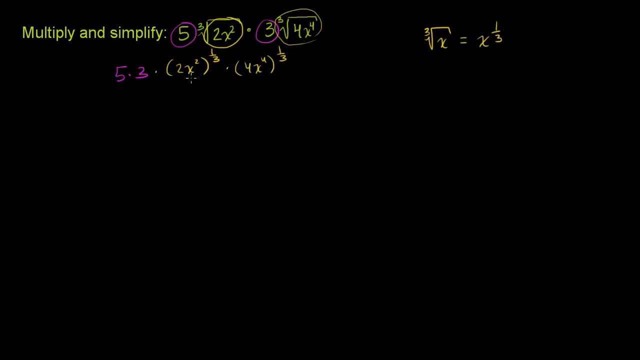 if we have two things that are both raised to the same power, and then we take the product, we could just take the product first and then raise it to the power. So if I have a to the x power times, b to the x power, 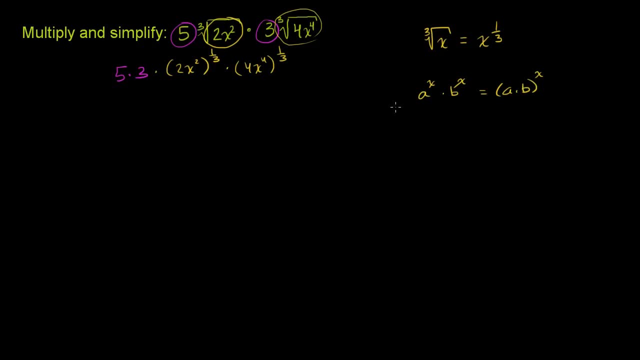 this is the same thing as a times b to the x power, So we can simplify This part of the expression right over here as 2x squared times 4x to the 4th to the 1 third power And of course 5 times 3, is 15.. 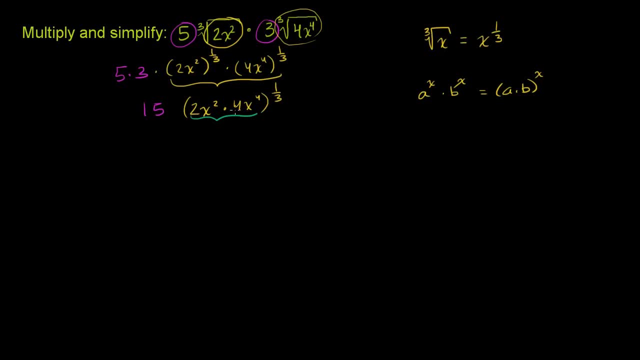 And if we simplify what's in the expression right over here, once again, it's commutative, so we can swap the order, And it's associative, and so we can swap the groupings. How we group them doesn't matter, because it's. 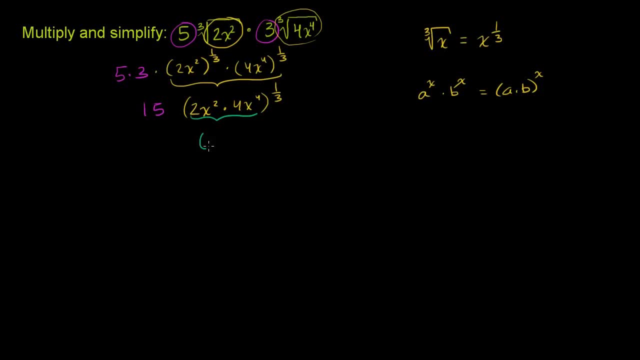 all multiplication here, This is 2 times 4, which is 6.. Times x squared times x to the 4th. x squared times x to the 4th is x to the 6th power, And it's all of that to the 1 third power. 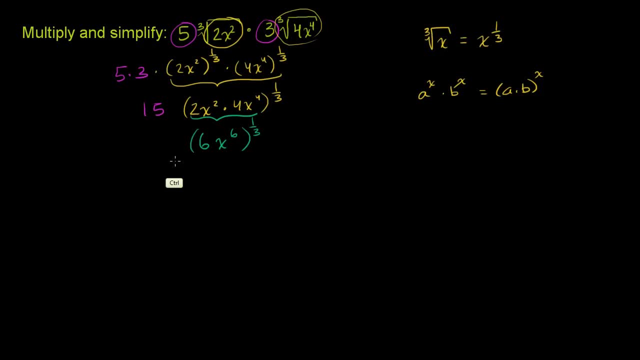 And then that is times that- oh sorry, not 6.. 2 times 4 is 8.. What am I doing? 2 times 4 is 8.. 2 times 4 is 8.. x squared times x to the 4th is x to the 6th. 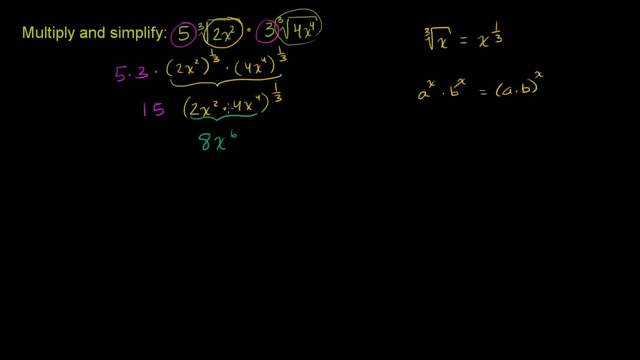 I think my brain was adding the exponents and wrote the 6 down. Of course, 2 times 4 is 8, not 6.. But we add the exponents. They have the same base: x squared times x to the 4th is x to the 6th. 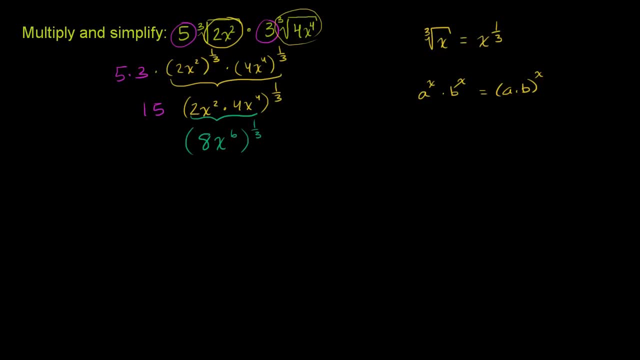 And we're going to raise that to the 1 third power, And then all of that is times 15. And then we essentially can use this property again- Actually, not that property. We know that, this, we know if I have something, well, actually, 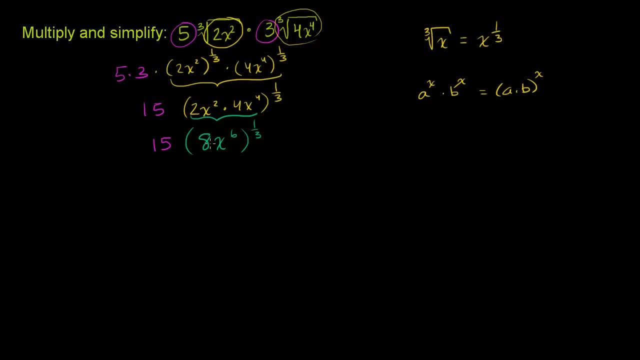 yeah, exactly this property. again We have something multiplied to a power. This is the exact same thing. This is the exact same thing as 8 to the 1 third power times x to the 6th to the 1 third power. 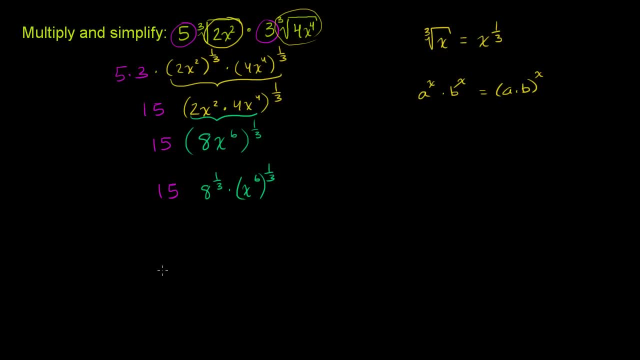 And then all of that is being multiplied by 15. And so 8 to the 1 third power, that's the same thing as the cube root of 8. You might recognize that 8 is 2 times 2 times 2..